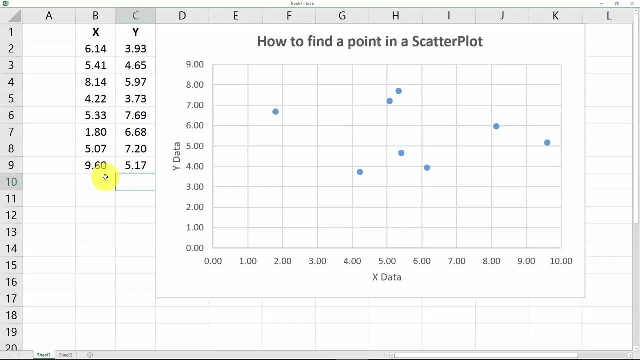 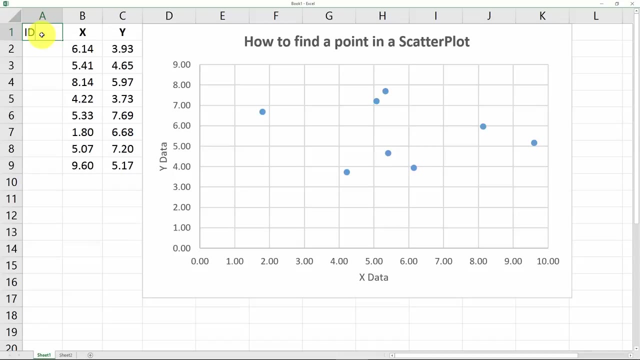 Now you probably want to know a better method, for what if I have hundreds of points and I need to identify one of them? what can I do then? So let me show you a little trick. Usually, when I have data like this: if it doesn't have an identification variable or 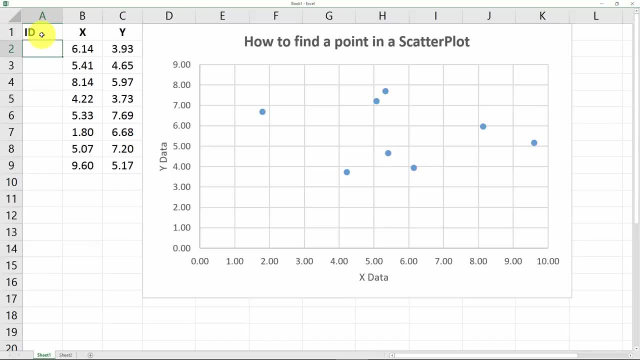 an ID variable, I'll create one, And so an easy way to create an ID, An ID variable, is just to number them one, two, and then you can highlight the numbers one, two, grab the little fill, handle down here and drag it down or double click it, and 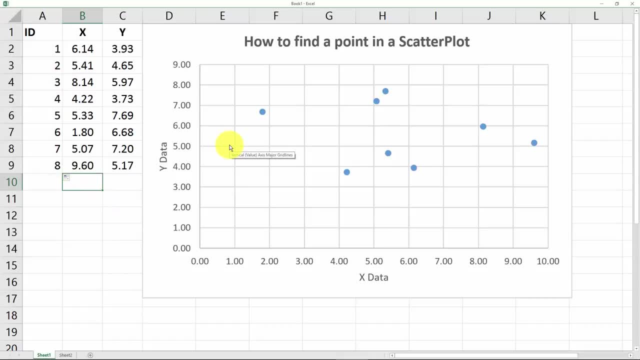 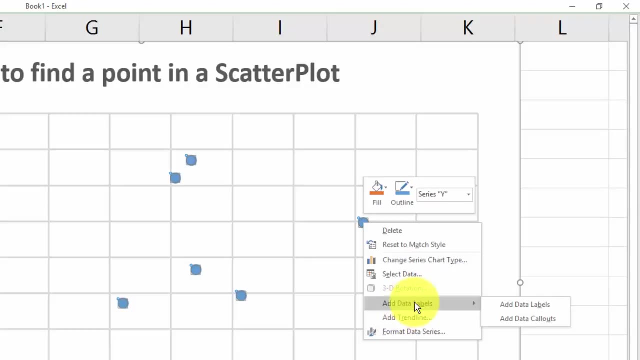 it'll fill down numbers and give each row a unique ID. Now how that can be used in a scatterplot like this is: if you right click on any one of the points in the scatterplot here, Let's go to add data, Add data labels. 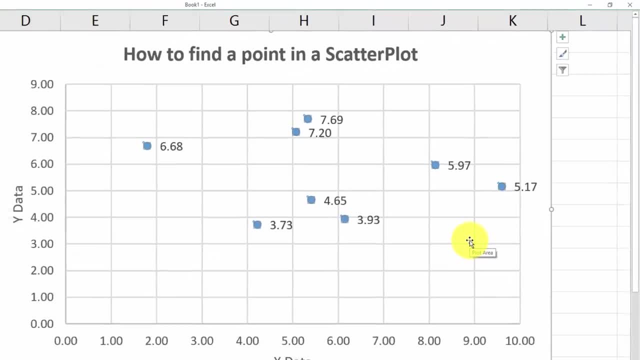 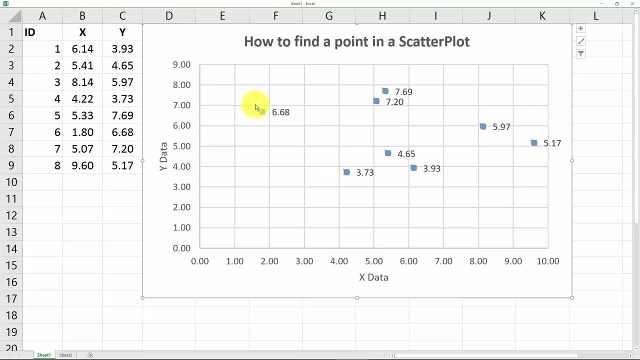 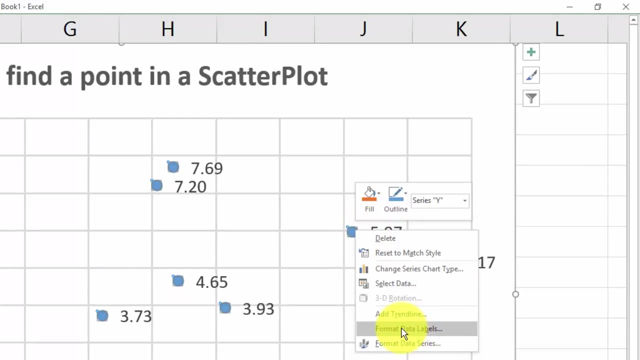 Add data labels And by default, what Excel wants to do is it wants to label it with the Y value. But that's not what we want. That's not going to help us here. So right click on that again and go to format data labels. 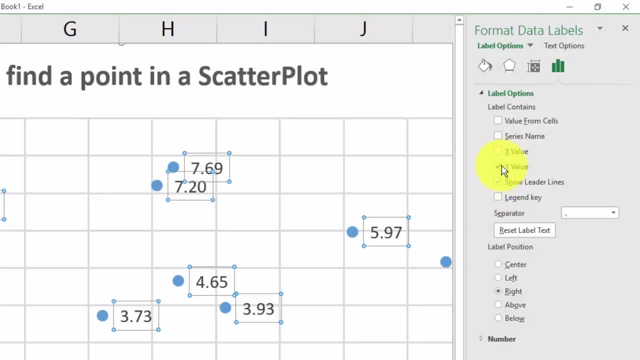 And here, instead of the little checkbox here, says Y value. What we want to do Is give it a label value from cells. So click that and it asks us, what data label range do we want to use? So click the little select button there and we want to select the numbers one through. 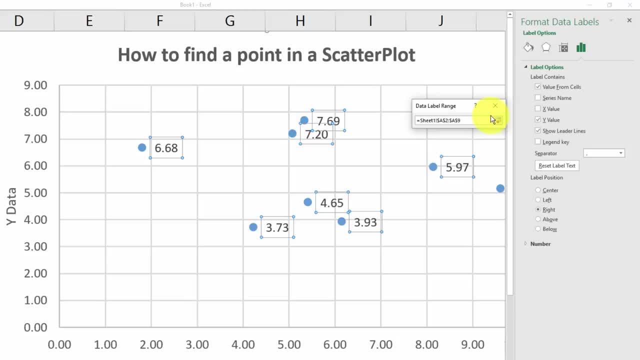 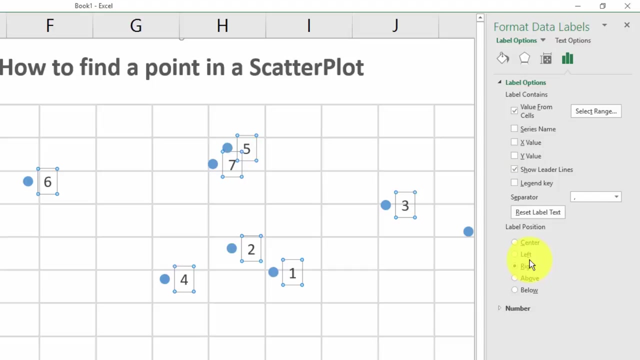 eight that we gave the data. Well, there's little labels that we created over here and then hit enter, Okay, Okay, And you see now that it has two labels. it has the ID number and the Y value. But if we go over here to the right side we can uncheck the box called Y value. 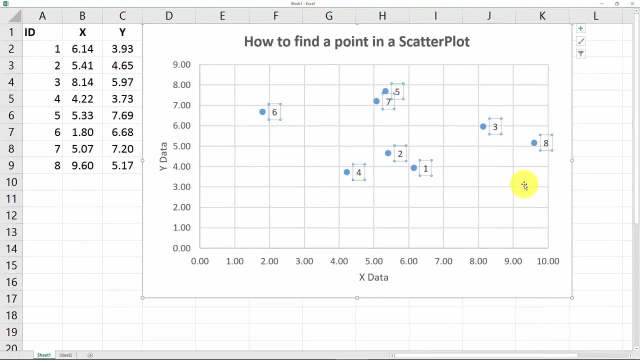 And now our, each of our data points are just labeled with that ID variable that we created, And I think in most cases that's going to be an easy enough way to be able to tell which point it is. And now we're going to go ahead and look at that one. 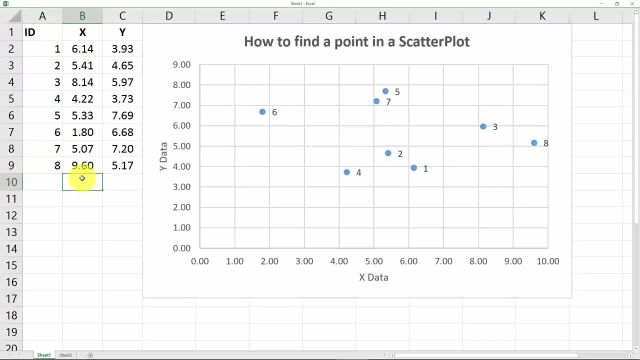 So, if we go back to our data, here's our data point. We're going to go over here and we're going to find the Y value And we're going to click on our data points. Okay, And we're going to see that our data points are not really in the right places to look.